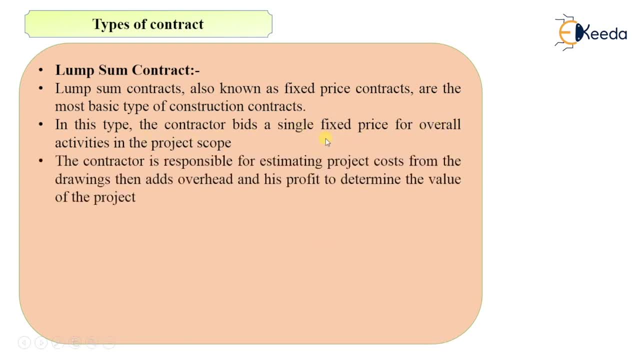 He will not mention the various rates of various items of work but he will mention or he will bid a single fixed price for the overall activities in the project scope And contractor is responsible for estimating the project cost from the drawings, then adds overhead and his profit to determine the value of the project. For example: 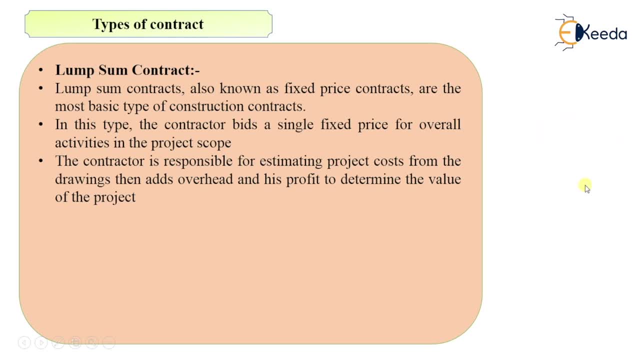 from the drawing, he will estimate the total cost of the project. For example, total cost of project is 10 lakh rupees and he wants 10% of the profit. The contractor wants 10% of the profit. So what he will do, he will calculate the estimated cost of the project. 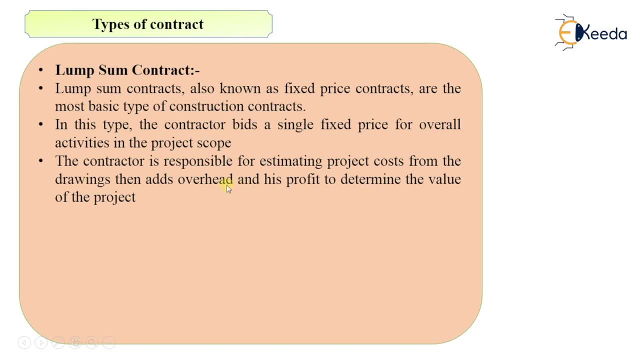 from the drawings and then he will add any overheads, if they are there, and his profit, For example, 10 lakh. I have given you the example, So he will quote 11 lakhs. Then he will add the total cost of the project as the quoted amount or a fixed amount or a fixed 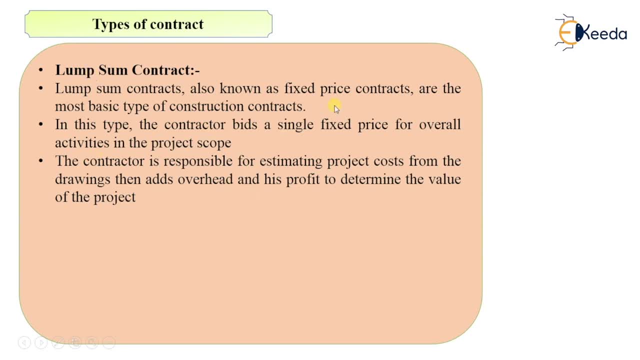 price for the overall cost of the project and that is called as your lump sum contract. Then all risks that are assigned to the contractor and there will not be any risk carried by the contractor. See what are the risks. for example, if there are chances that material prices will. 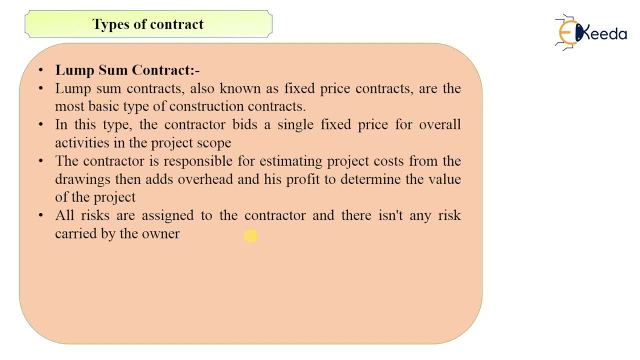 increase or they're at side. There are certain conditions that may occur. unforeseen conditions, unforeseen circumstances will be there, contingencies will be there. so there are some risk involved in the execution of work but totally the contractor will be responsible for for that and there will not be any risk by the owner, as he has already. 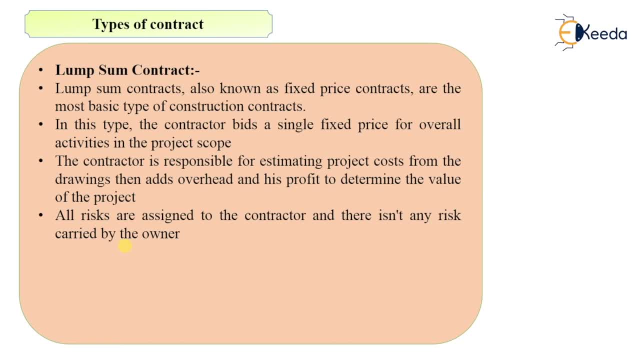 quoted the total amount he will be paid for. as i have given you the example that contractor already quoted that i will complete your work in 11 lakh rupees, so there will not be any extra charges he will mention- he cannot mention extra charges after that, so there will not be any risk to the owner. 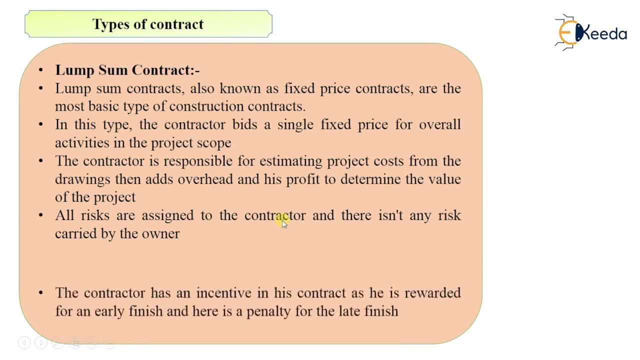 and there are certain risks that will be assigned to the contractor and the contractor has an incentive in his contract as he is rewarded for early finish and there is penalty for late finish. there will be incentive given to the contractor if he finishes his work early and there will be penalty given to the contractor if he finishes. 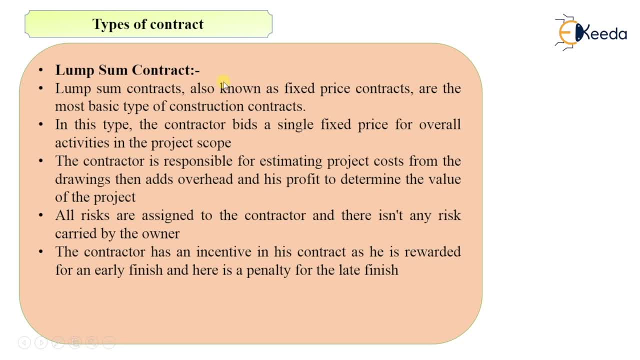 the work later. remember this: in case of lump sum contract, then this contract is ideal when the project scope is well defined at the design stage, because there is limited flexibility for modifying the design during the construction period. this type of contract can only be used, or should be- 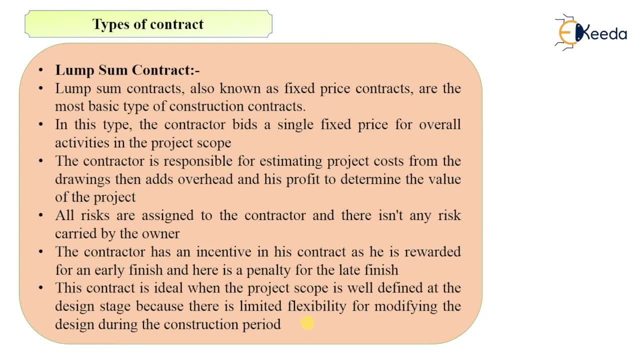 used only when the project scope is well defined. and the project scope is well defined when the design is finalized. there are no chances that design will be changed because- see, the total amount has to be mentioned before starting of the project now. so that's why this type of contract. 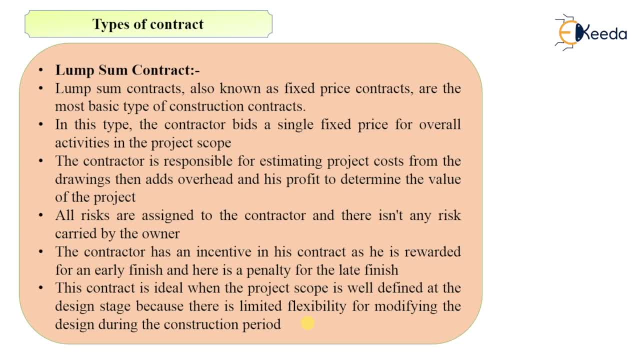 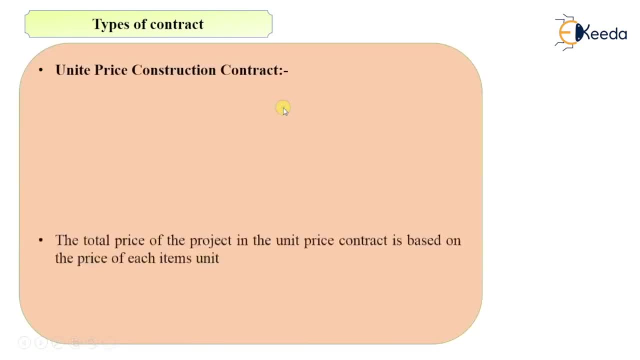 should be used. if the design is fake- there are no chances of changes in the design- then in that case you can use the lump sum contract. then there is another one unit price construction contract. see: the total price of the contract is 1.5 lakh rupees and the total price of the contract is 1.5. 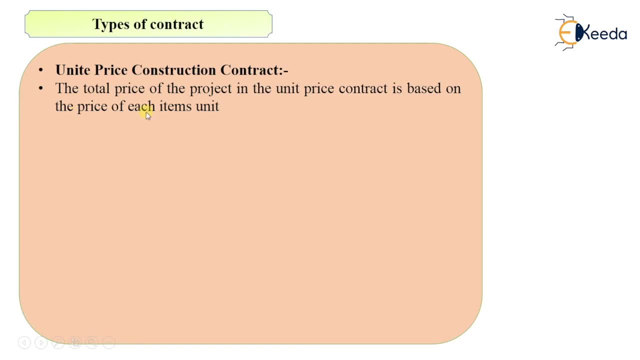 lakh rupees and that's all the money. now the total price of the project in unit price contract is based on the price of each item of work. see in the previous slide. we have seen lump sum contract. the total amount of the whole project will be bid by the contractor. but in this type of contract 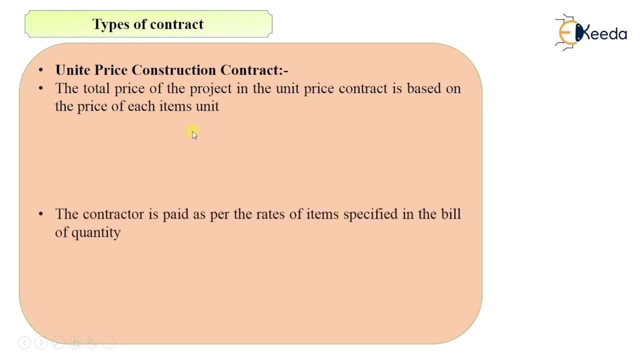 the total price of the project in unit price. contract will be based on price of each unit or each item of the work and contractor is paid as per the rates of items which are spaces- terracotta- specified in the bill of quantities. he will mention each and every items: rate, items, price. 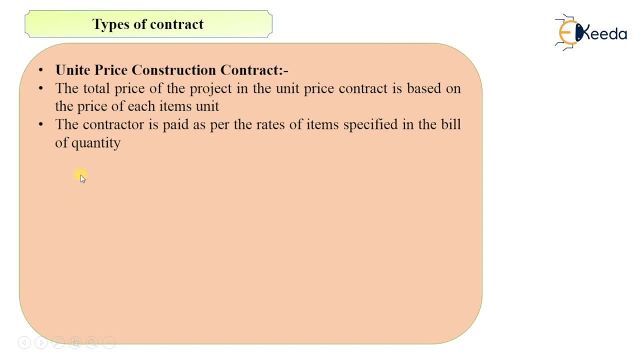 in the bill of quantity and as per that he will be paid. so in such case the risk will be shared, with both contractor as well as the owner. both will share the risk that i told you in the previous slides. what are the possible risk contingencies then? this type of contract is more flexible for. 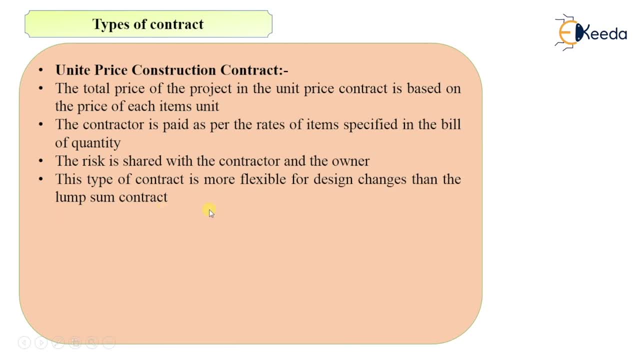 design changes than the lump sum contract because, see, in lump sum contract amount is fixed. there are no chances of changes in the design. but in case of unit price construction contract, there are chances of changes in the design. there is a scope of change in the design, the construction of the. 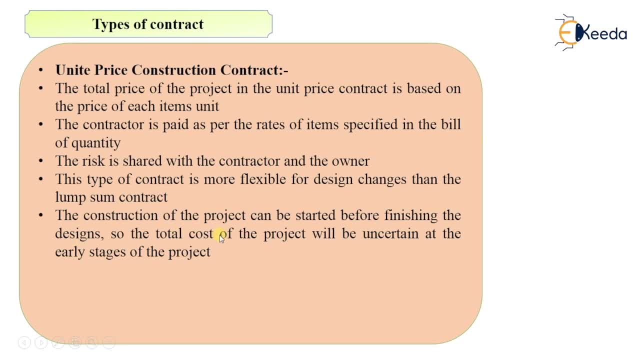 project can be started before finishing the designs. so the total cost of the project will be uncertain at the early stages of the project. see, even before finalizing the design, you can start the work because this type of construction project, this type of contract, is that contract that can be started before the finalizing of the final cost. therefore, 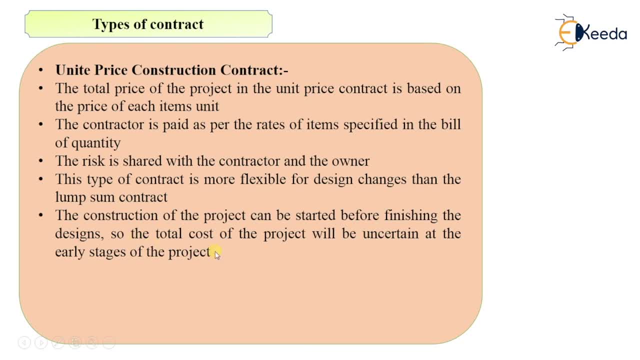 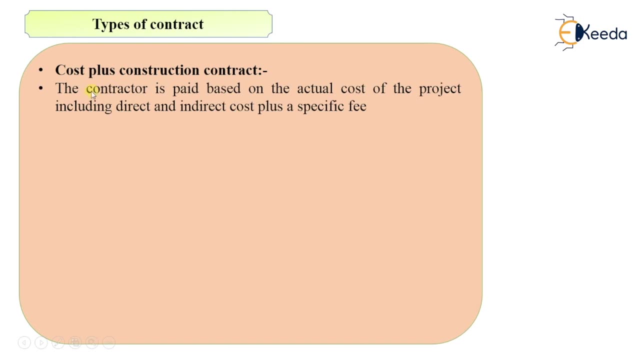 before completion of the project there will not be known or final cost will not be known. before the final, before starting the work or in the early stages of the project. then we have cost plus construction contract- see contractor- is based based on the actual cost of the project. 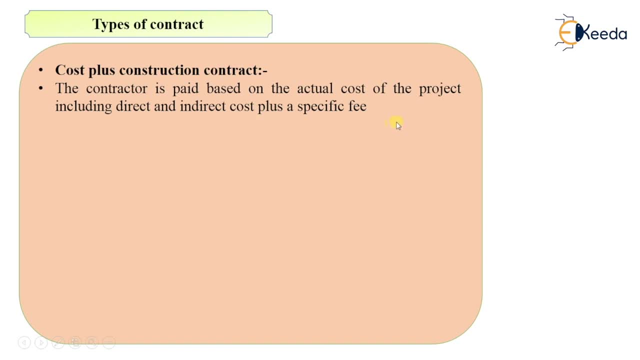 including direct and indirect cost plus a specific fee, as i told you the in the previous examples that, for example, a contractor is taking a work, he is executing a work for a owner for an owner and the cost of the project is 10 lakh rupees, so obviously he will charge more. 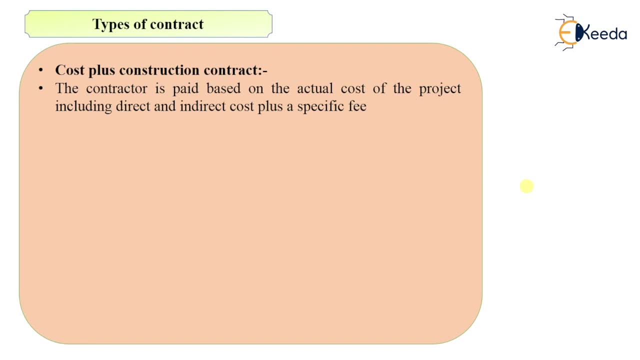 for his profit. let us consider that profit is 10 percent, so the total cost of the project will be, and lack, the original cost of the project plus 10 percent profit. that is one lakh rupees. so the total cost will be 11 lakh rupees. so that is. 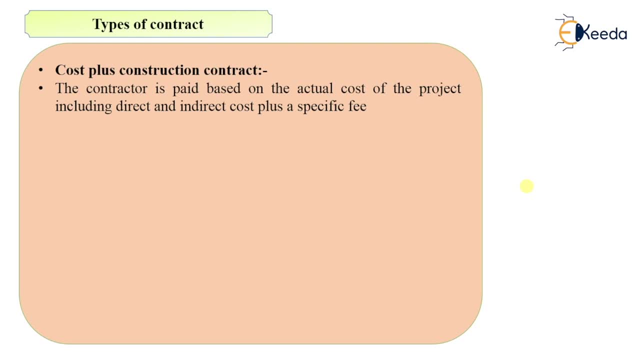 nothing but your cost plus construction contract. the contractor will be paid. how much he will be paid? actual cost of the project plus direct and indirect cost and a specific fees. They will include direct cost, indirect cost plus there will be certain specific fee that will be provided to the contractor for the completion- maybe his profit. 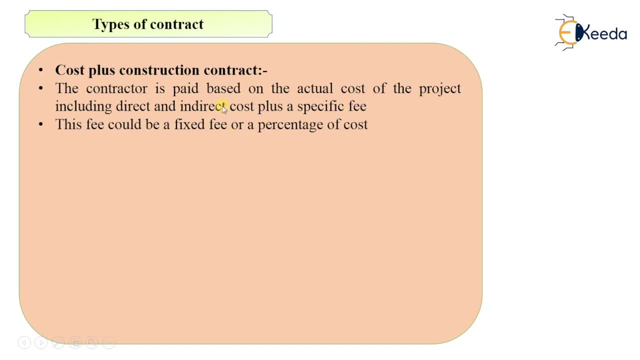 So that fee can be in the form of percentage or they that can be in the form of fixed amount, As I told you. if it is a percentage, for example contractor is saying I want 8%, whatever is the cost of the project. for example, cost of project is 20%, so 20% or 20 lakh rupees. 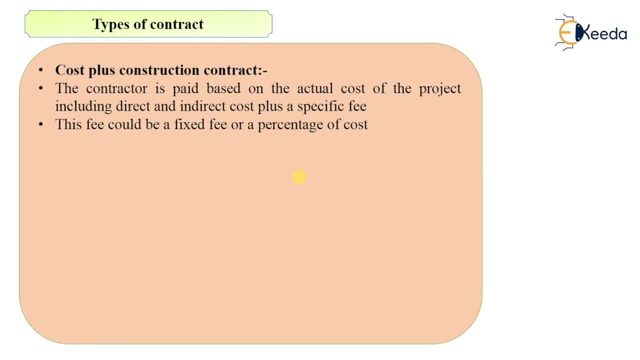 for example, the total cost of project. So 8% of 20 lakh rupees will be given to the contractor in addition to that original cost. And if he is saying that for a 20 lakh cost or for the project of 20 lakh rupees cost, 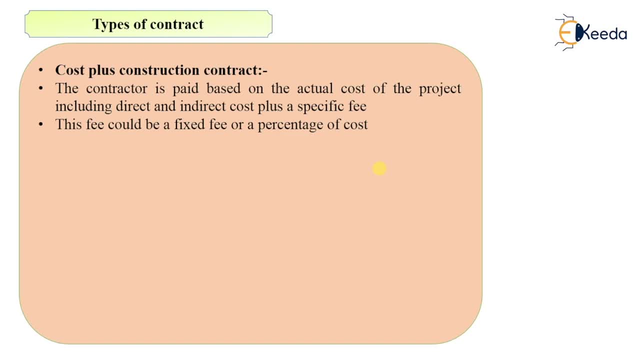 I will take extra 2 lakh rupees So that can be also be given. So it will be paid either a fixed percentage or a fixed fee in this type of contract And all risks are assigned to the owner and he gets involved with the contractor in the 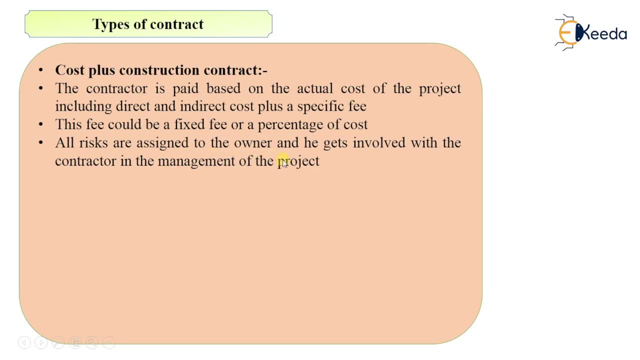 management of the project. All the risks will be assigned to whom? to the owner, and he will be involved in the contractor management processes of the project and all that. he will be involved with the contractor and contractor has no risk in case of increasing the cost of the project because, see, he knows. 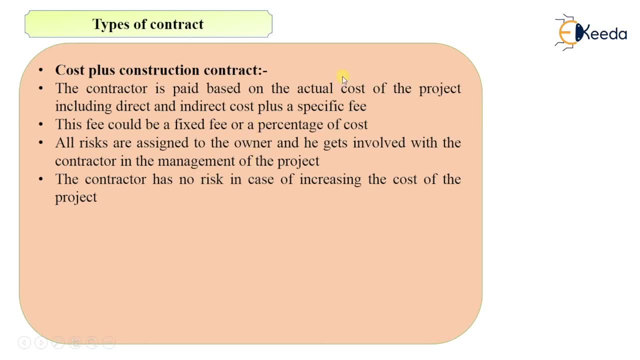 that he will definitely get a fixed amount or fixed percentage. for example, the cost of project is in the initial stages. it is found that cost of project will go about 10 lakh rupees. So 10% of 10 lakh rupees will be given to the contractor. 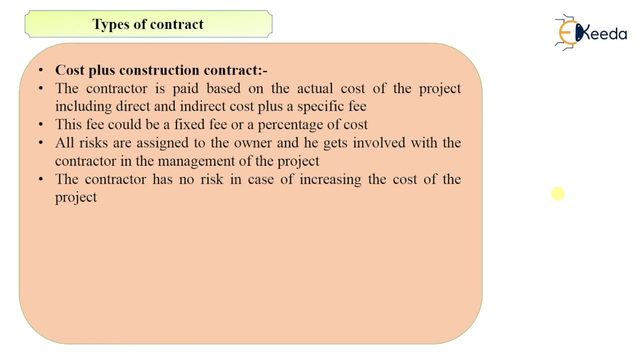 And if owner is thinking that let us use some high quality material, So the total cost of project goes 1 lakh 12 lakh rupees instead of 10 lakh rupees. So what contractor will get? he will definitely get 10% of 12 lakh rupees. 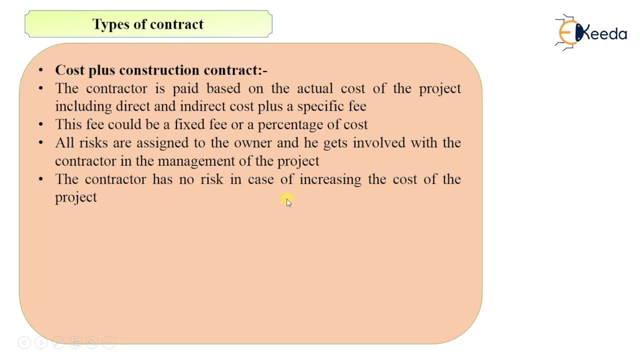 So he will get whatever is the amount. so there is no risk associated with the contractor. Also, there isn't any incentive for any arrangement. There is no incentive for any early finish. he will not get any incentive if he is finishing the project earlier. 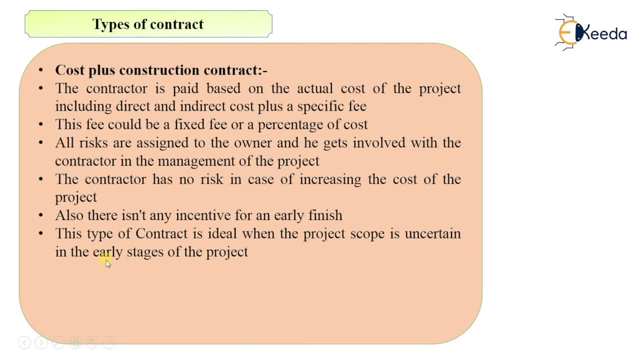 And this type of contract is ideal when the project scope is uncertain in early stages of the project. As I told you, this type of project or this type of contract can be suited well suited when there is uncertain scope of the project in the early stages of the work and the contractor 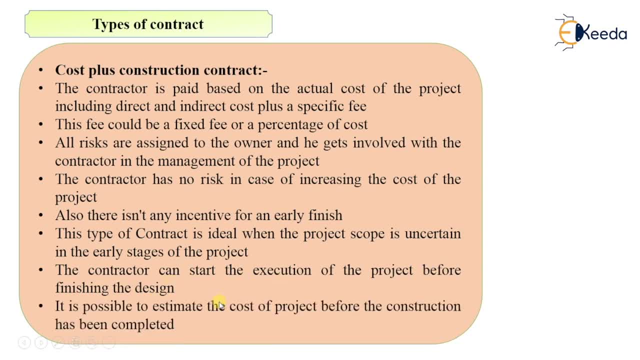 can start the execution of project before finishing the design. also, And it is even possible, It is possible to estimate the cost of project before the construction has been completed. Before the construction of project, you can estimate that how much will be the probable cost of the project. 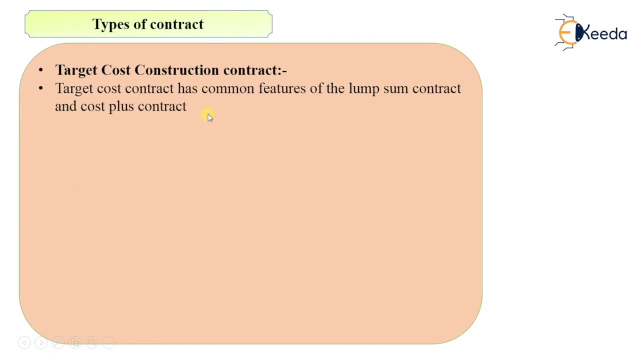 Then we have target cost construction contract. What is it See? target cost contract has common features of lump sum contract and cost plus contract. It will have features of both. What features Lump sum contract is the lump sum amount given, And cost plus contract will be some fixed fee or fixed percentage.